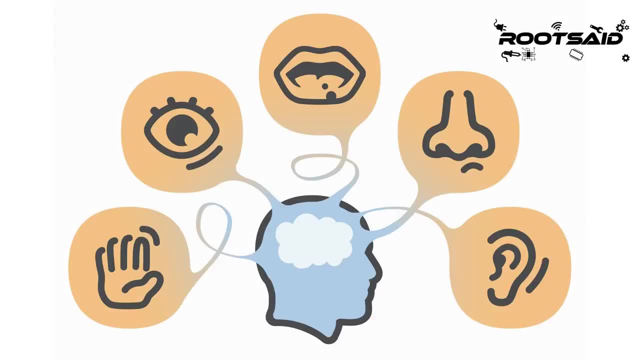 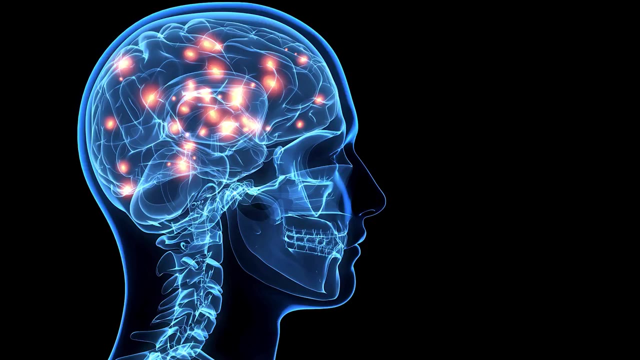 other organism, like a human being, We have sense organs. We see things with our eyes, we hear things with our ears, feel things with our skin, taste with our tongue and smell with our nose. Our neurons transmit these signals from our senses to our brain, where we process them, Our brain. 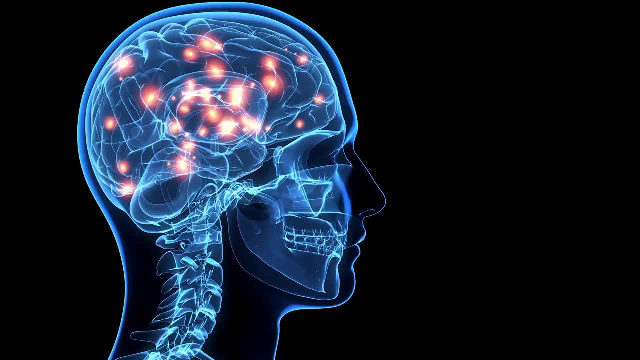 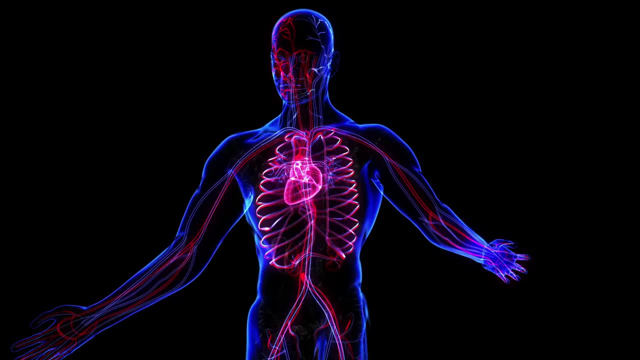 processes these signals from these sense organs, takes decisions and sends signals to your muscles to move your hand, legs or do whatever you want. Then we have a heart that circulates blood, supply oxygen, provides energy for the working of our entire system. 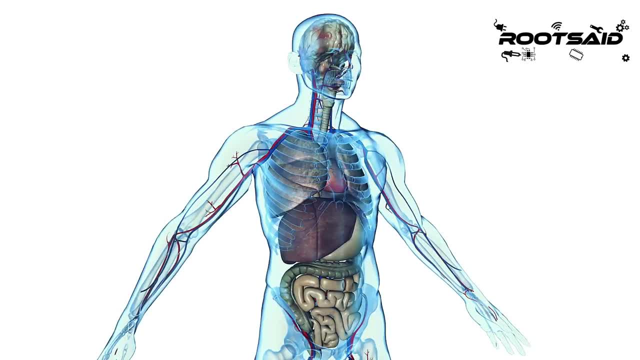 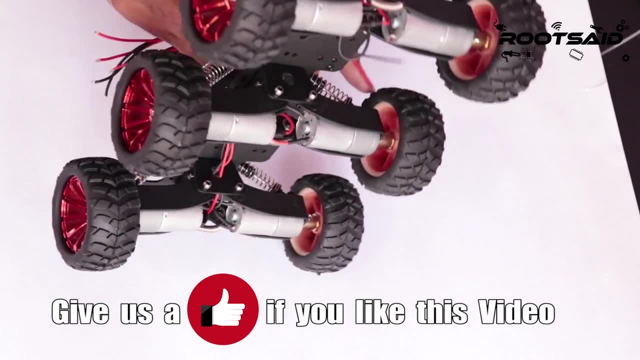 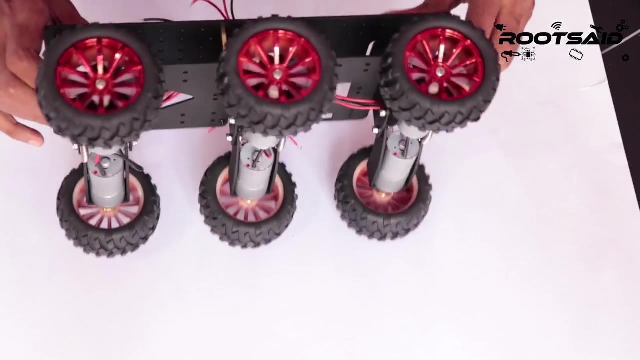 We have a body where the sensors, muscles, hearts, veins and all other parts are neatly assembled. This is same as in the case of a robot: The robot chassis or the body of the robot. A robot have a chassis or a robot frame which is similar to our body, A frame that will support the whole robot. 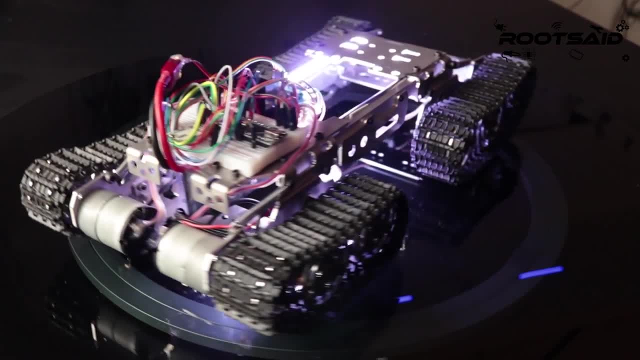 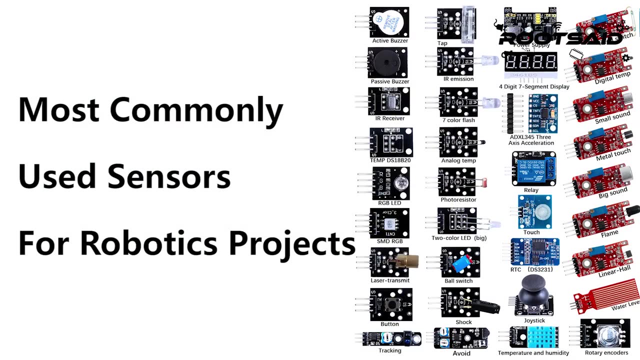 A frame which is having enough space and is capable of handling the weight of all the sensors, our source and all the cables used in the robot. Then we have the sensors, or the sense organs. A robot have sensors, such as IR sensors, which will sense infrared rays, ultrasonic sensors to sense ultrasonic rays. 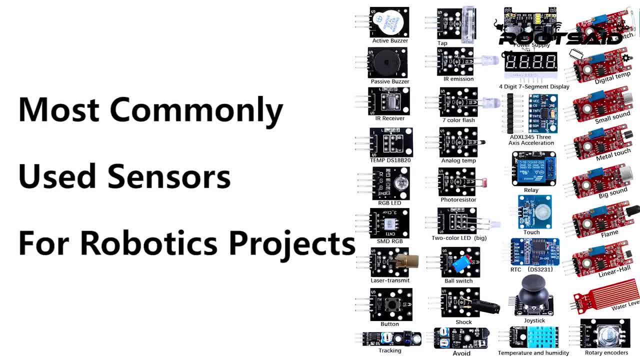 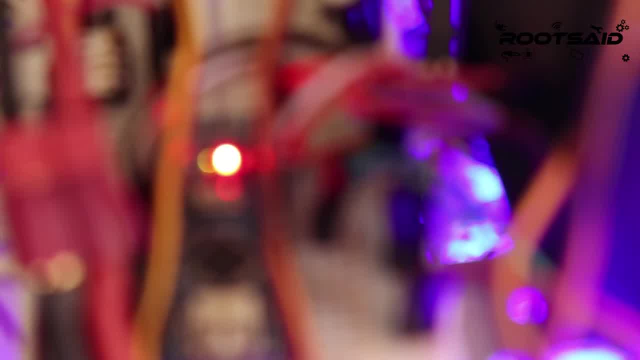 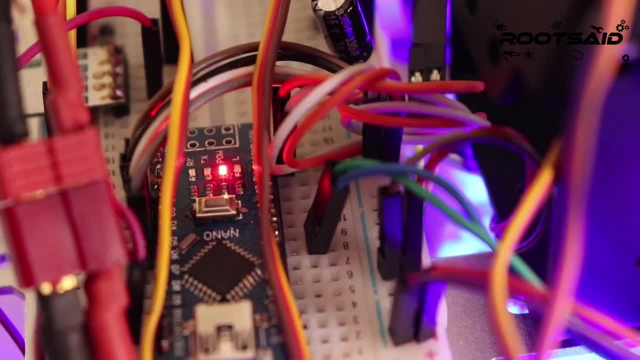 heat sensors to sense temperature, pressure sensors to sense touch or pressure, and so much more. Next, we have the brain. We now have all the data from the sensors. Now, what to do with this sensor data? We need to process it. For that we will need a 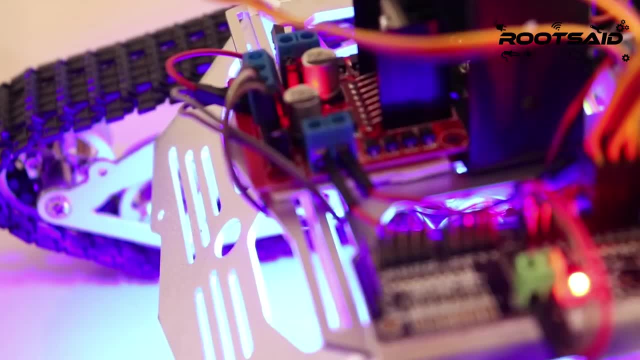 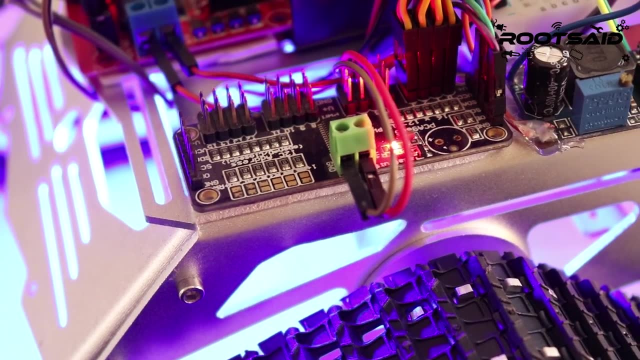 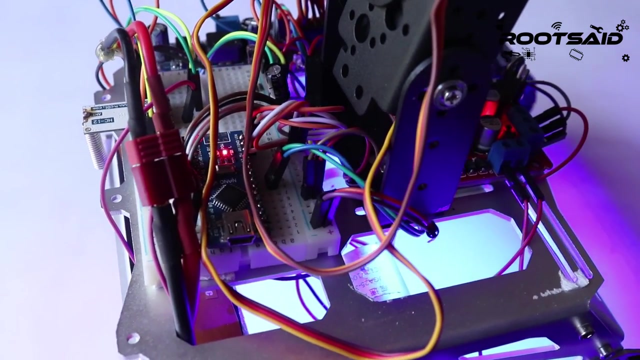 single processing unit. Normally, we will use a logic circuit. This can be a simple circuit consisting of resistors, capacitors, transistors to perform simple logical decisions, or a micro controller such as Arduino or a PEG that can perform complex calculations. That totally. 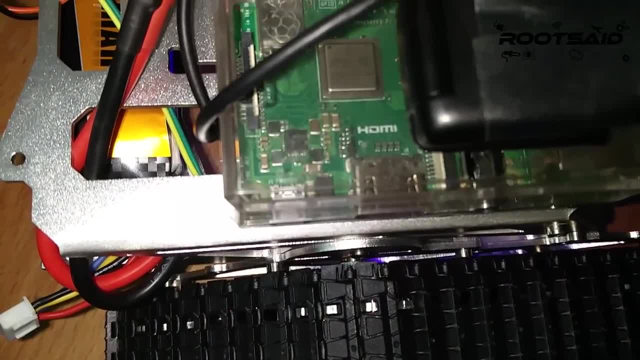 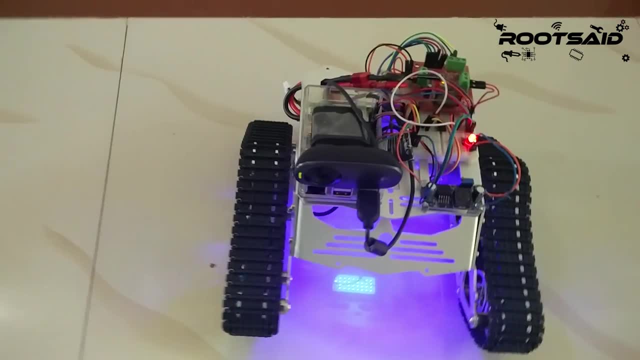 depends upon the complexity of your robot. Arduino and Raspberry Pi are the most commonly used controllers in the field of robotics. I will talk about Arduino and Raspberry Pi, their differences, similarities, and what they can do and cannot do in the next video, so that you can choose the.